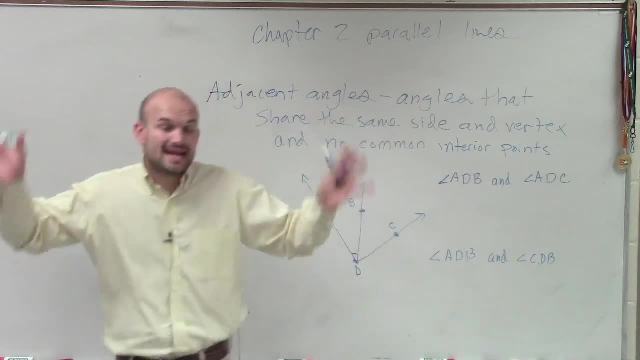 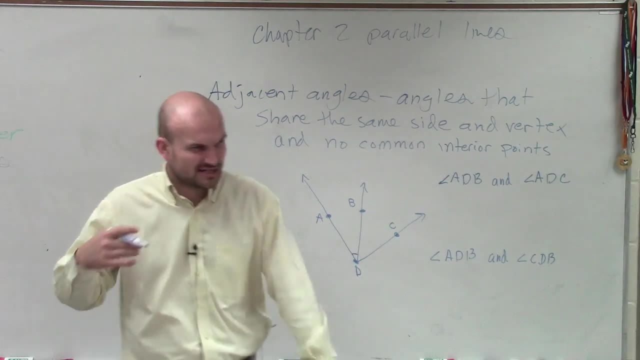 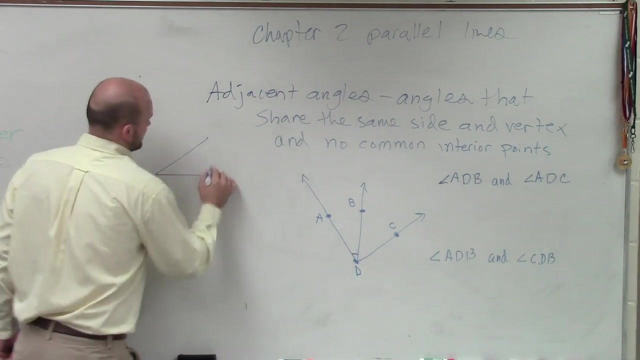 That's angle ADB. That's angle ADB. Now notice, on angle ADB, there's a couple characteristics I want to remind you guys of. First of all, angle ADB has a vertex. of what, Guillermo? What is the vertex of ADB, You remember? Okay, let's go back to it. An angle contains a vertex and then two sides. 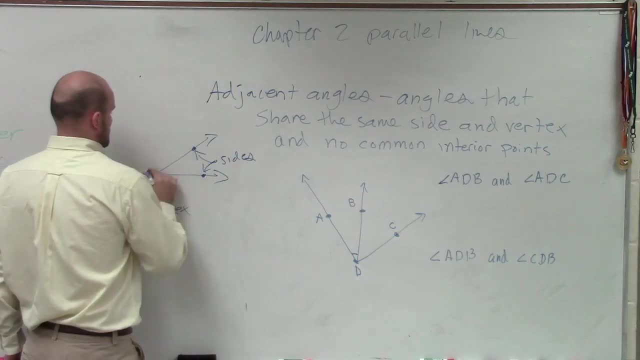 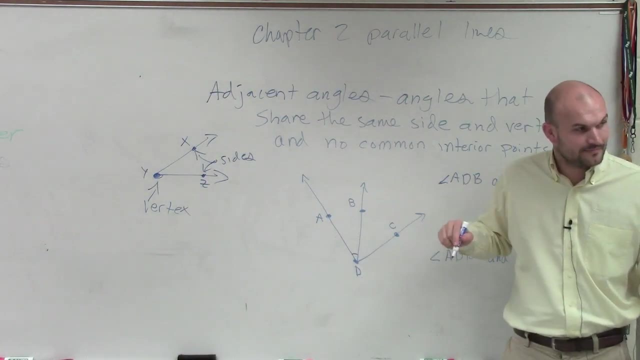 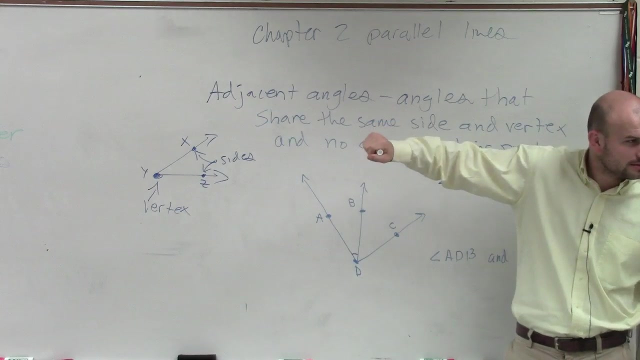 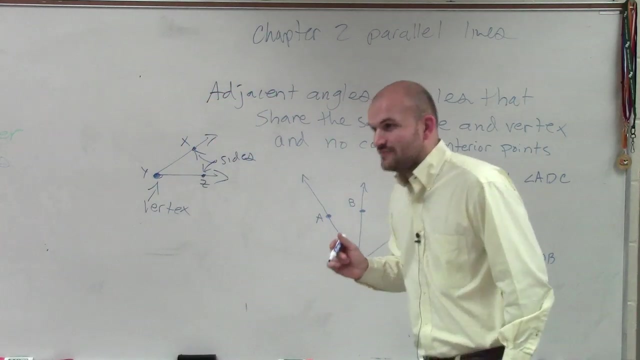 So, Guillermo, what is the vertex of ADB, ADB, What is the vertex of that angle? Which one? D, Exactly Right? The vertex is where the two rays come together. Yes And Josh, do you remember what a side is of that angle, ADB, What some side would be of this angle? 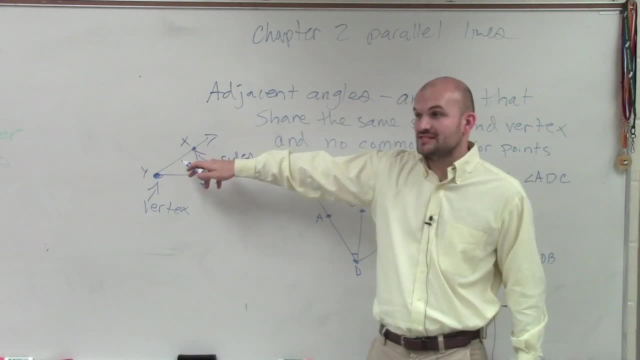 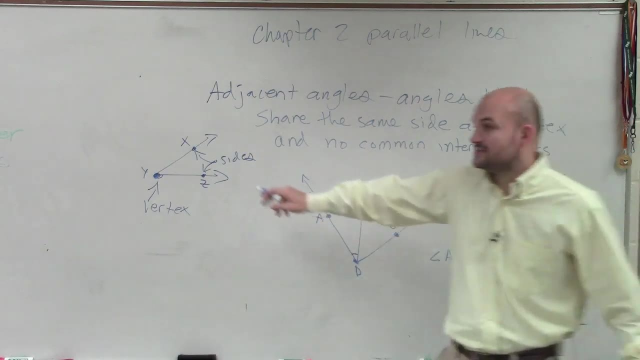 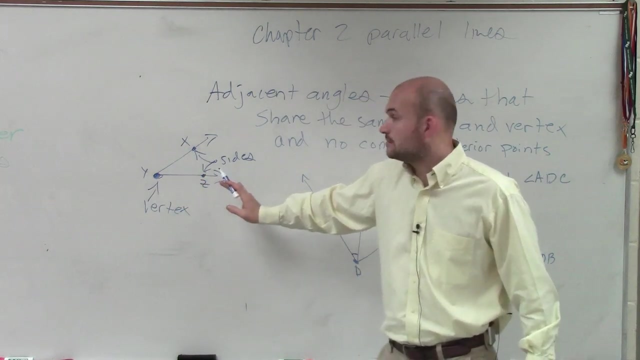 Do you know what the sides are of this angle? Here the vertex is Y. What is the length of my two sides? What are my two sides? Do you know? No, No, Do you know what the sides are? What would be a side X and Z? Yeah well, those are points on the sides. But how do we label the sides? Yes, 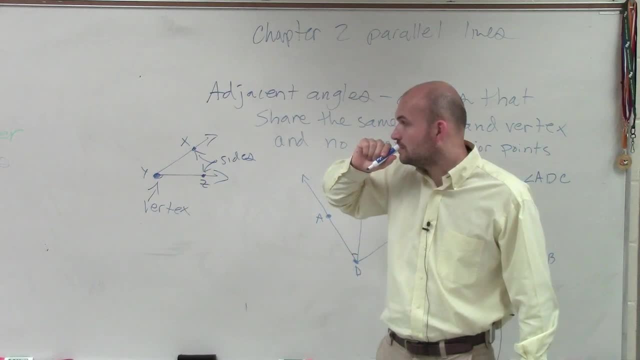 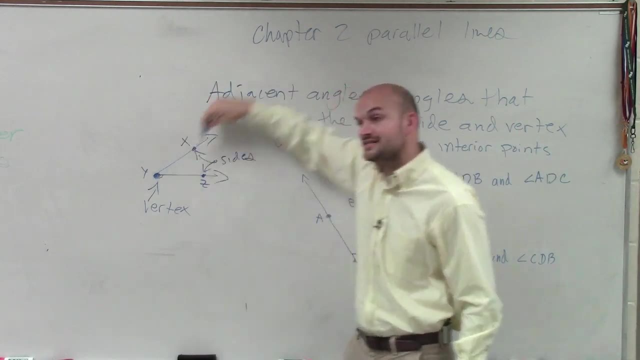 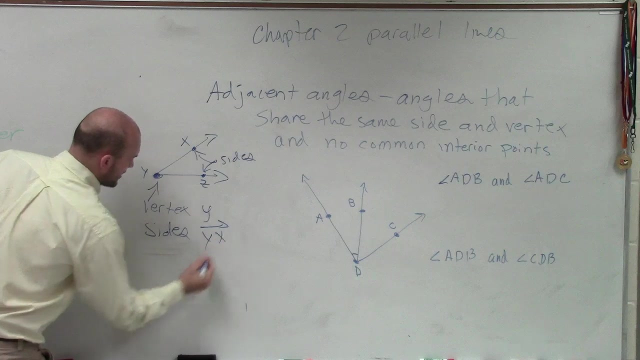 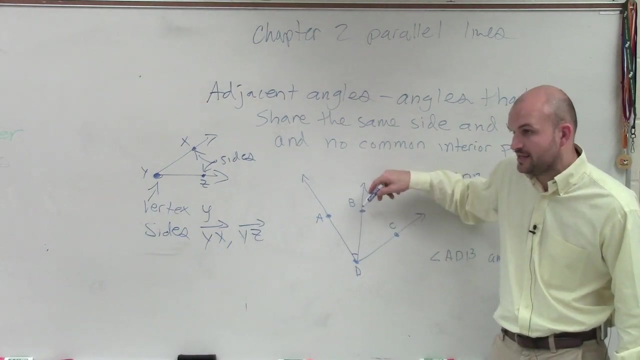 Y, X, Y and then Y, Z. Right, You always want to go from the vertex To the other point. So, yes, X and Z are on the sides, but that's not the name of the side, because the side is a ray. So we would say the vertex is Y and the sides are YX- they're a ray, and YZ, which is a ray. Right, All of you guys on your homework, a lot of you messed up on that, so I made sure you guys did that correctly. Now, Josh, going back to this, what's a side here? What is a side for my angle? ADB. 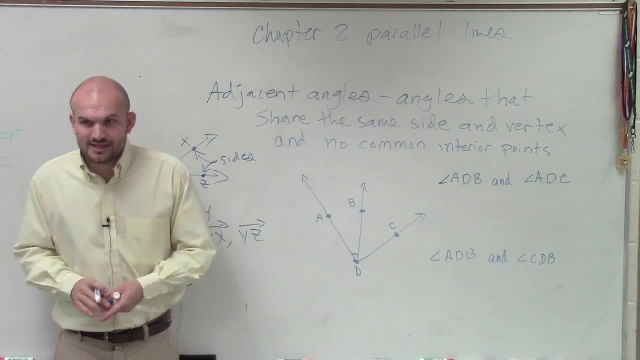 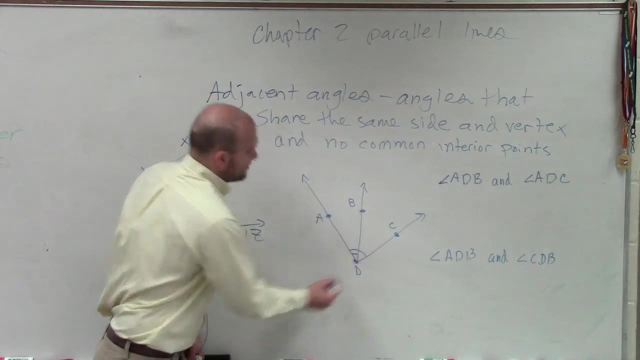 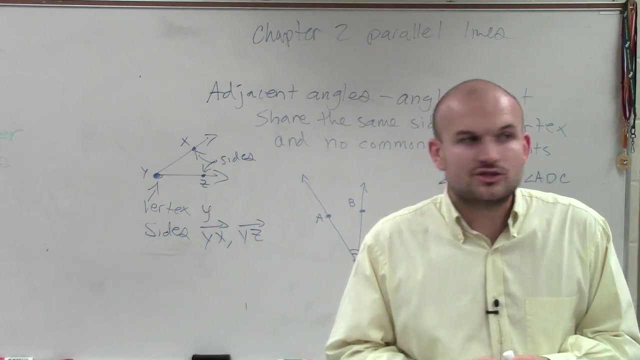 DA, exactly Now. let's go and take a look at. the other angle Is ADC. you guys can see ADC. that's this big angle right here. So you have ADB and ADC Out of those two angles. what side do they share, Alana? do you know What side does ADB and ADC share? 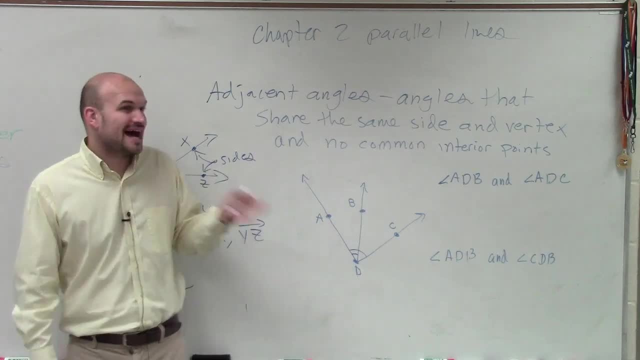 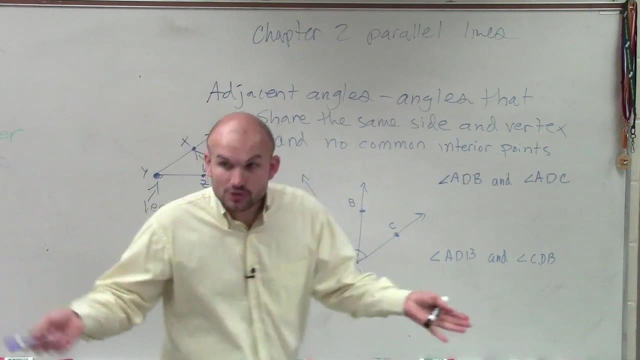 A, Well, A is a point. so what side, though? Remember side is going to be a ray? What DA DA, right? So we made sure we labeled it from the vertex to the point. So yeah, they share a side. Yes, Yes. 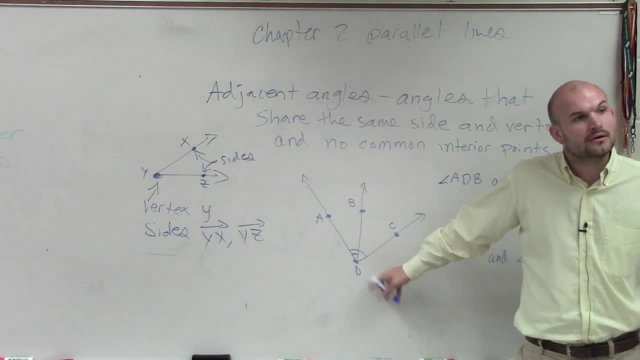 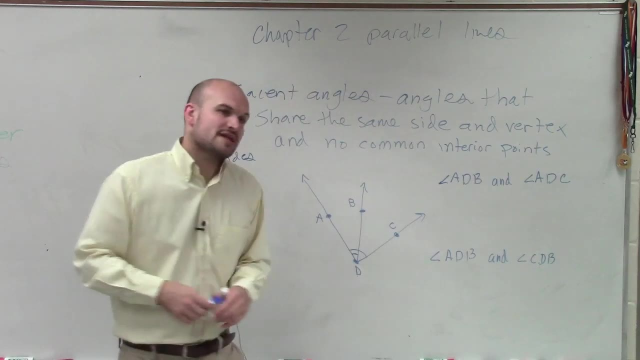 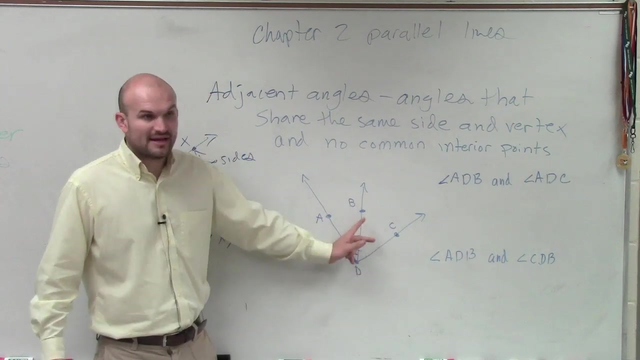 And do they share the vertex? Do they have the same vertex? Okay, So that's a possibility, right? Let's go and take a look at the other two angles. So these two share a side and share a vertex. Now let's look at the angle ADB and CDB. 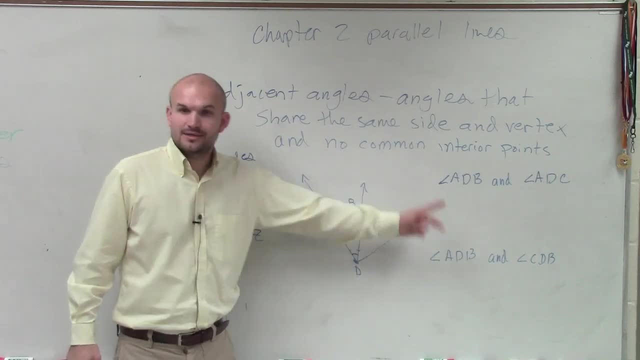 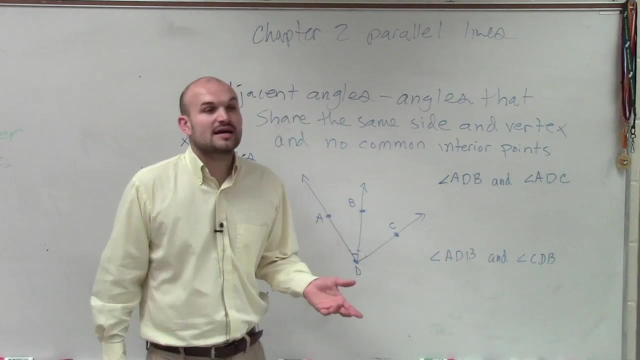 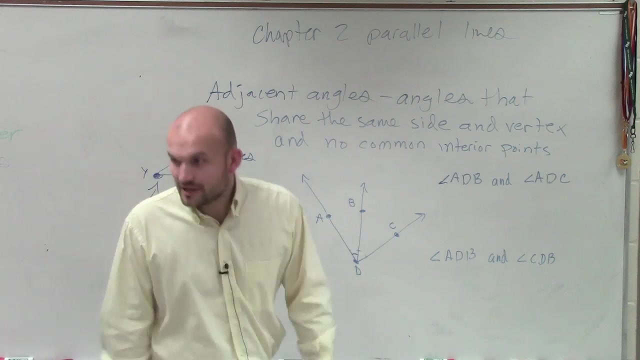 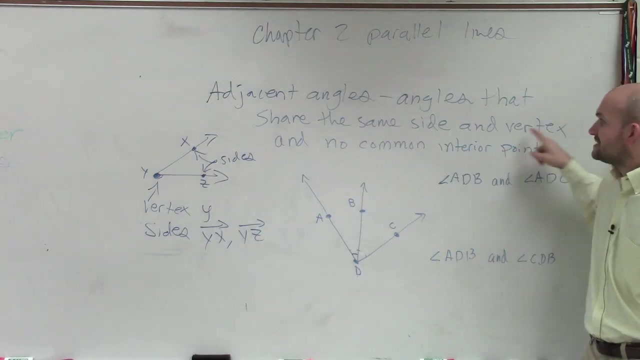 ADB, CDB, ADB, CDB. What do ADB and CDB? do they share a vertex? Yes, Which vertex? D, D. Do they share a side? Yes, Which side? DB, DB, Very good. So, ladies and gentlemen, right now we have two examples, Both examples, ow. both examples share a side, share the same side, and they share a vertex. 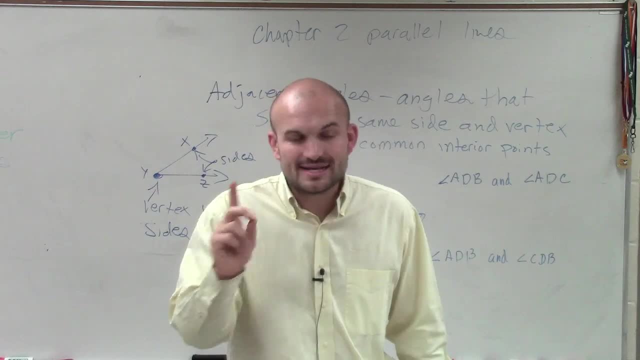 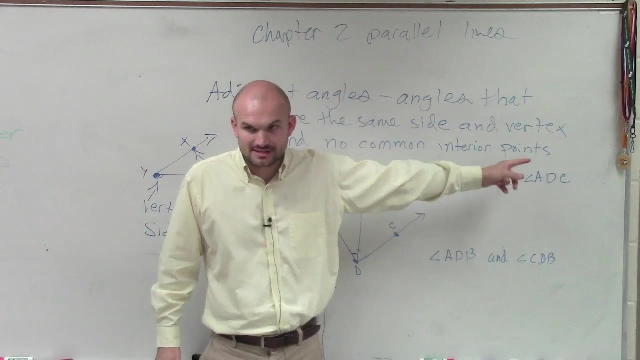 So they both could be adjacent angles. but I'll tell you, only one is an example, and one of them is a vertex. It's a non-example, And the difference comes in is they share no common interior points. Alright, let's look at these two examples. 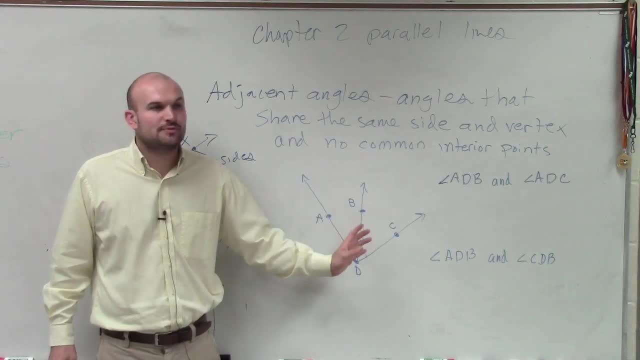 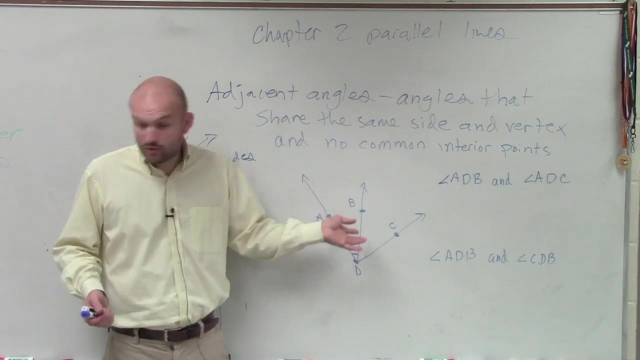 Does the angle ADB and CDB? do they share any other points inside of one another? or are they just right next to each other? They just well. what point do they share that's inside of their triangle, inside of their angle? 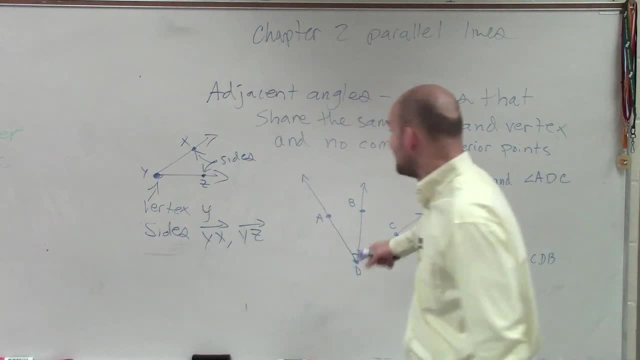 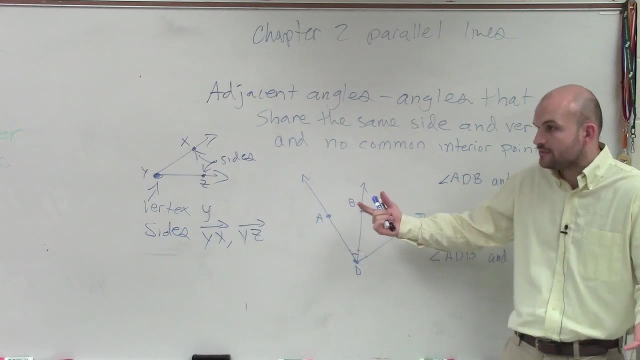 B, B, though well, B is not actually inside, though. It's on the line that they share, Right, so it's not inside this angle. ADB B is not inside of it. it's a part of it, right. 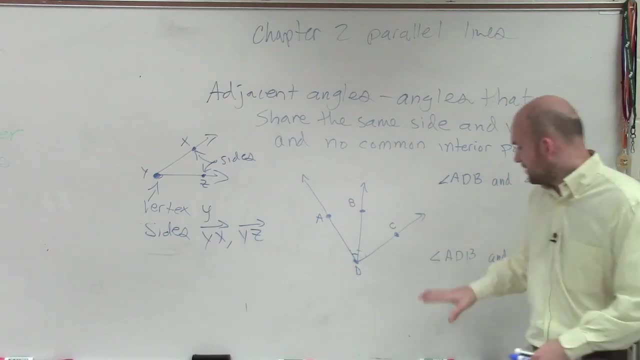 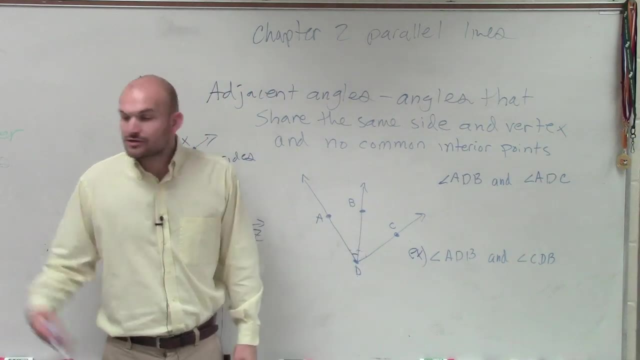 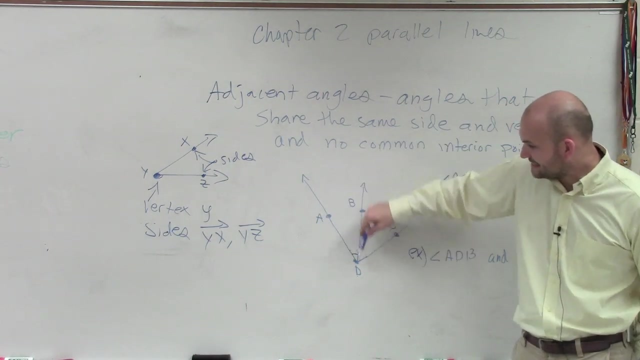 And CDB. B is a part of it as well. So therefore, since they don't share any common points, that is our example. So let me talk about B. why B is inside our other angle? If I'm looking at this, I have ADB and then ADC. 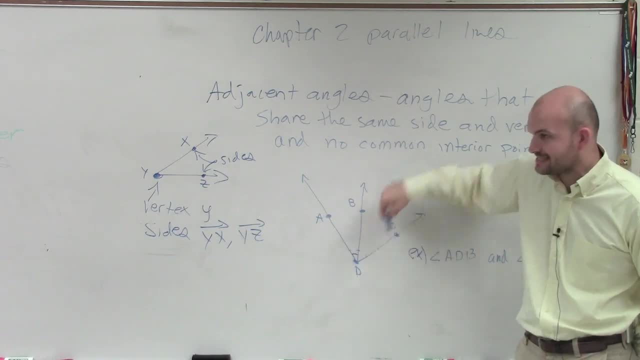 Do you see how the point B is inside the point ADC? Does everybody see this? This is very important for everybody to look at That ADC, by point B, is inside of it. Therefore, they share a common interior point. So this is what we call a non-example. All right.